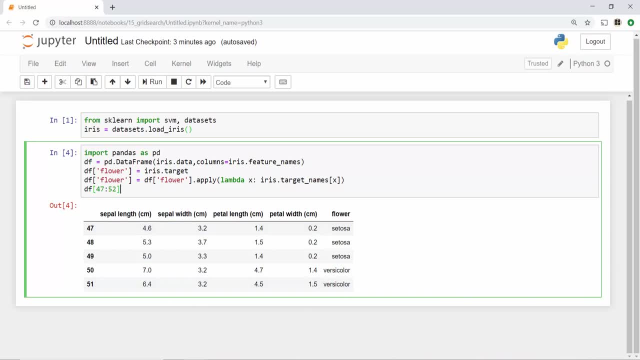 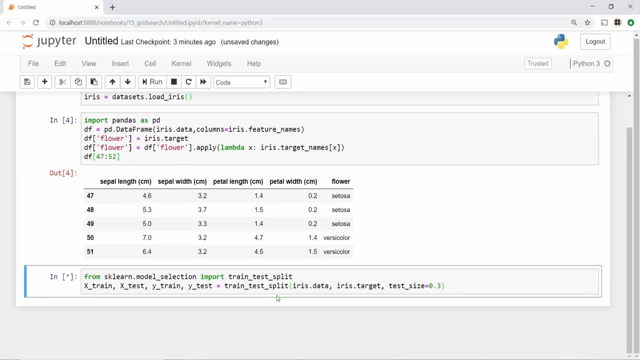 being shown in a table format. The traditional approach that we can take to solve this problem is that we have to choose the model that we are going to use. We use train test split method to split our data set into training and test data set. Here I'm using 7030 partition. and then let's say: we first 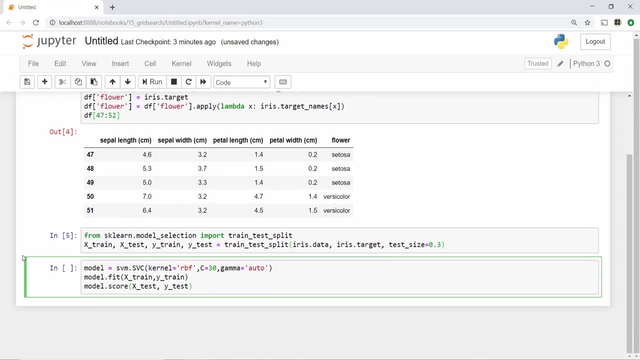 try SVM model. First I'm going to show you how to do hyperparameter tuning and then we'll look into how to choose the model. Just assume that you are going to use SVM model and using SVM model you can train the model and you can calculate the score. Here I randomly initialized these parameters. I. 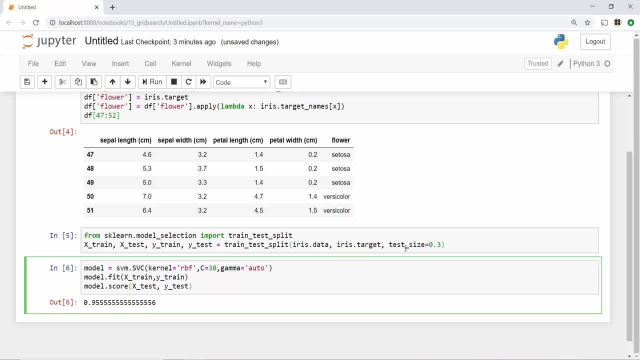 don't know what is the best parameterI'm just going with some value. The issue here is that based on your train and test set, the score might vary. Right now my score is 95%, but if I execute this again, X train, X test into samples are going to change, so it will change from 95 to now. 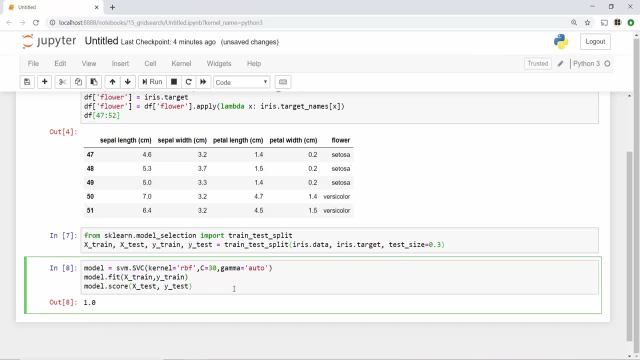 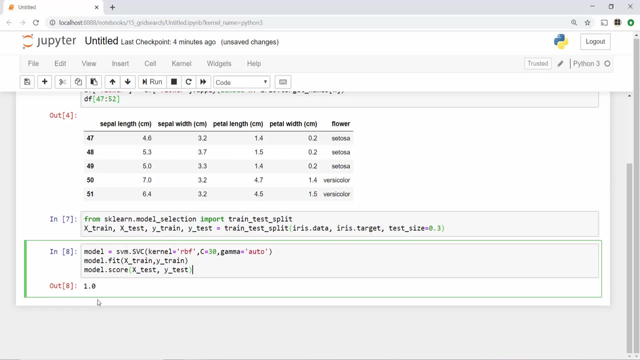 change to 1.. I cannot rely on this method because the score is changing based on my samples. For that reason, we use k-fold cross validation. I have a video on k-fold cross validation, so if you want to pause here and take a detailed look at it, you can. 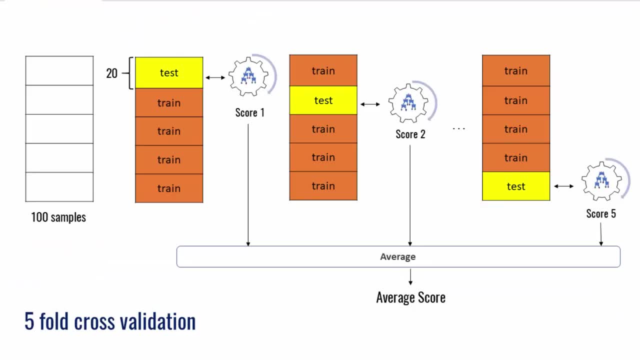 go there, but I will just give you an overview. As shown in the diagram, what we do in a k-fold cross validation is we divide our data samples into n number of folds. Here I am showing five folds and we take five iterations. in each iteration, one fold is test set and the remaining 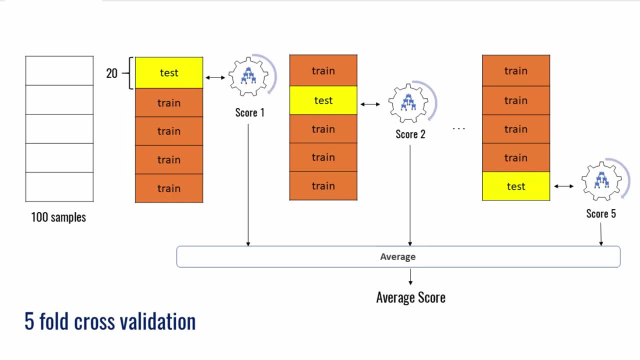 is our training set and we find the score for that iteration and we take these individual scores from each iteration and we make an average. This approach works very well because you are going across all the samples okay and we have a method called cross well score which can. 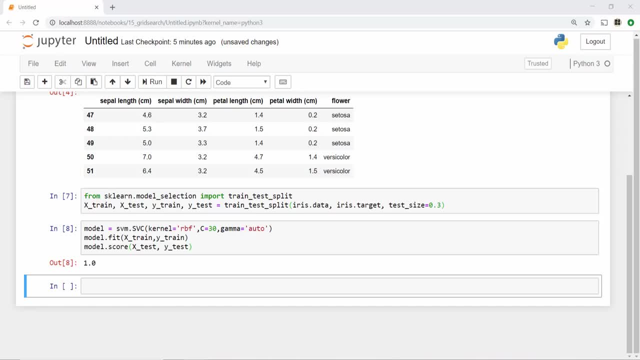 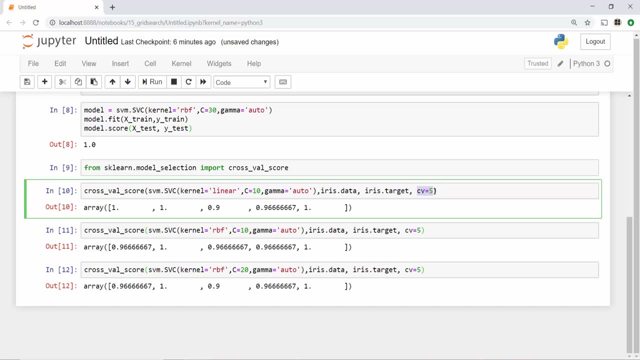 determine our Ск score. you will see for each iteration. we willAlso take three pendulum circles, three formulas and one tell you the score of each iteration here what i have done is tried cross well score for five fold. so cv is equal to five, means five fold, and tried this matter on different values of kernels. 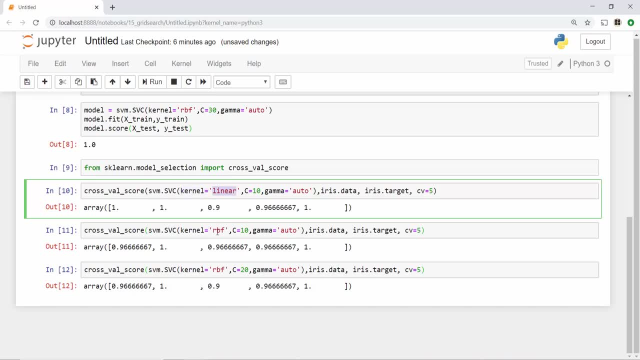 and c. okay, so here kernel is linear, here it is rbf, c10 and here c is 20. for each of these combinations i found the scores, so these are like five. you can see there are five values here and these are the scores from five iteration. you can take the average of these and find out what is. 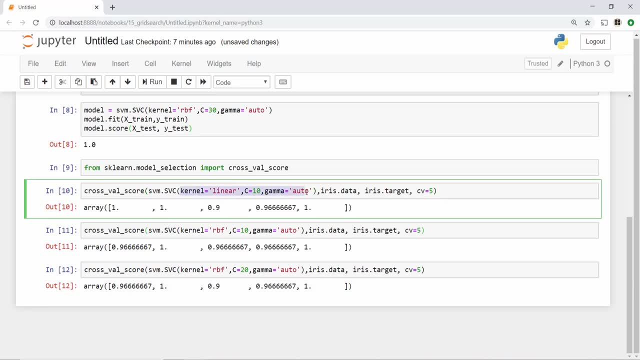 your average score and based on that you can determine the optimal value for these parameters. but you can see that this method is very manual and repetitive because there are so many values you can supply as a combination of kernel and c. right c could be one, two, three hundred. so for how? 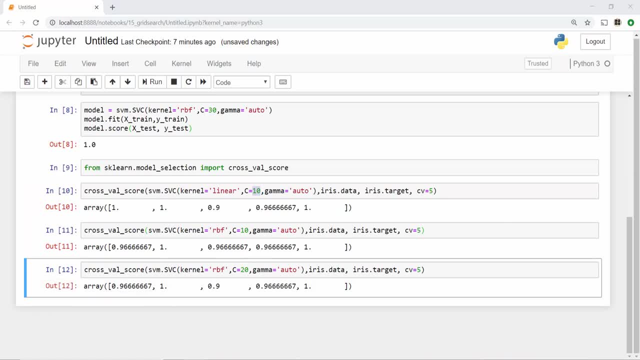 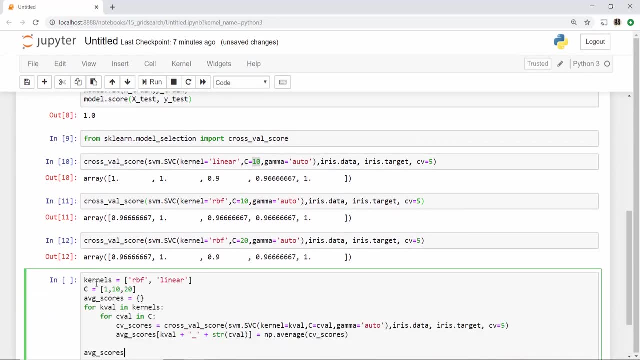 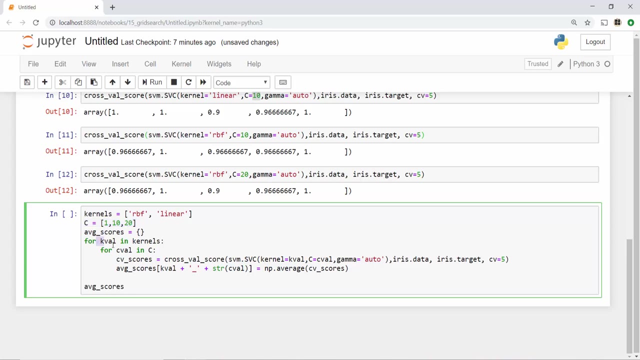 many times you're going to write this line. so the other approach you can take is you can just run a four loop. okay, so i'm doing the exact same thing, but using a for loop, so i have my possible values of kernel and then c, and then i ran a for loop on both of this and i'm supplying those values here. 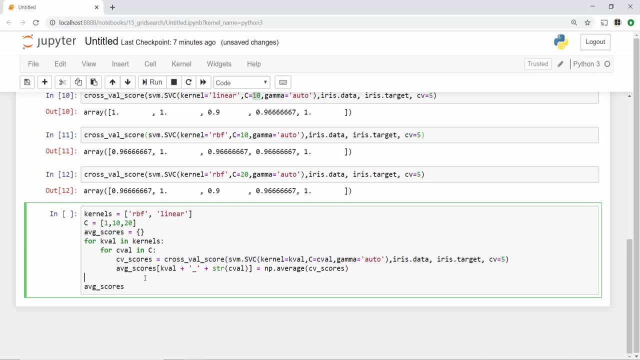 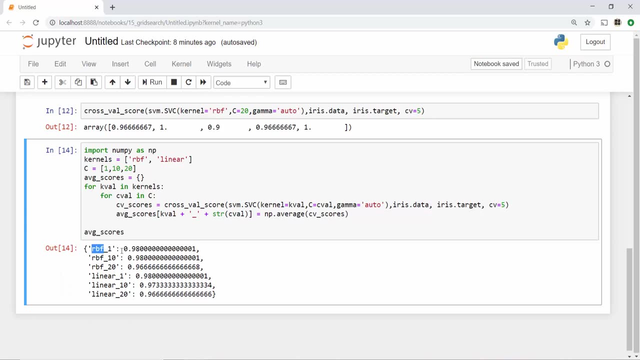 you can say c here, k well and c well, and then find the average scores right. when i execute this, i get these scores okay. so with rbf and one, the score is this. rbf and 10, the score is this, and so on. just by looking at the values, i can say that rbf one and the value of c being either one or ten. 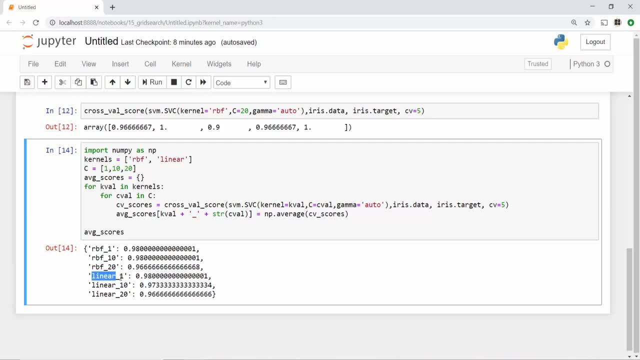 or linear kernel, and c being one, will give me the base score. you can see that these scores are low, so this way i can find out the optimal score, uh, using the hyper parameter tuning. but you can see that this approach also has some issues, which is if i have four parameters. 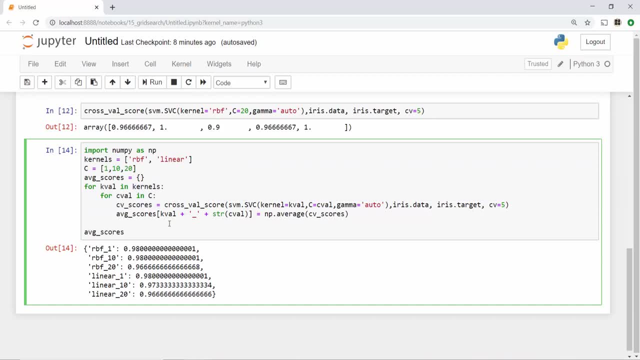 for example. then i have to run like four loops and it will be too many iterations and it's just not convenient. luckily, sklearn provides an api called grid search cv, which will do the exact same thing. okay, so grid search cv is going to do exact same thing as shown in this code here in line number. 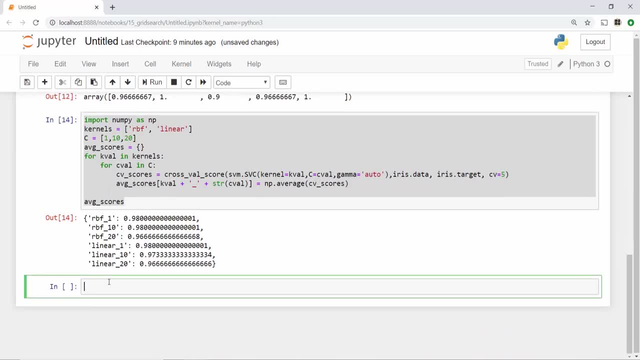 14. all right, so i'm going to do the same thing, but you will not that we will be able to do that in a single line. so i'm going to do the same thing, but you will not that we will be able to do that in a single line of code. okay, so the first thing you do is you import grid search cv from sklearn model. 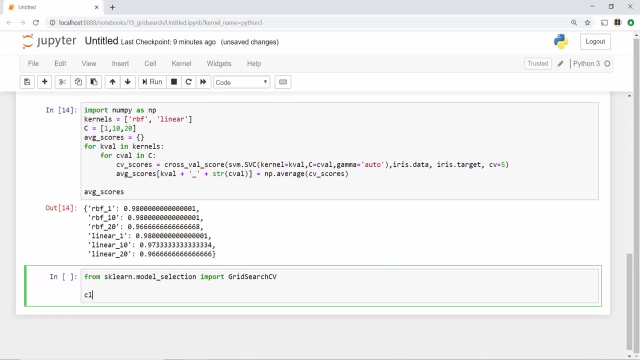 selection and then we will define our classifier. the classifier is going to be grid search, cv, where the first thing is your model. okay, my model is svmsvc. i'm supplying gamma value to be auto. if you want gamma to be in your parameters, you can do that. okay, but for this example, i'm just 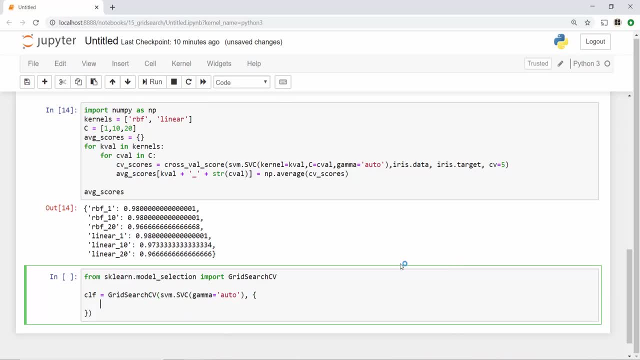 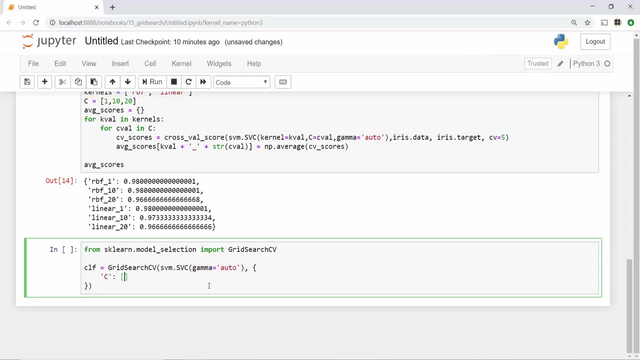 keeping it static. now, the second parameter is very important. second parameter is your parameter grid. okay, in parameter grid you will see, i want the value of c to be 1, 10 and 20.. okay, these are like different values that you want to try. the second parameter is kernel and you want to try the. 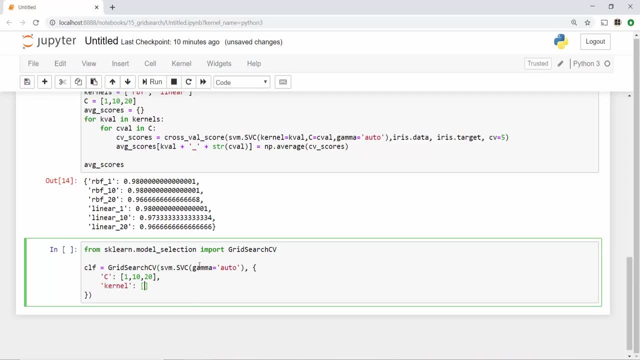 kernel and you want the value of your kernel to be rbf and linear. okay, so these are the two values. there are other parameters in grid search cv, for example, how many cross validations you want to run. grid search cv is still using cross validation. okay, it's just that we are making this particular. 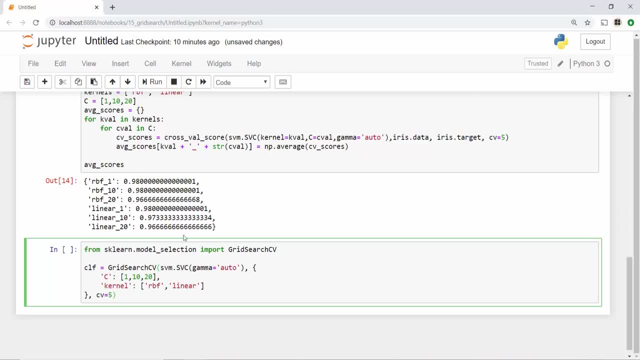 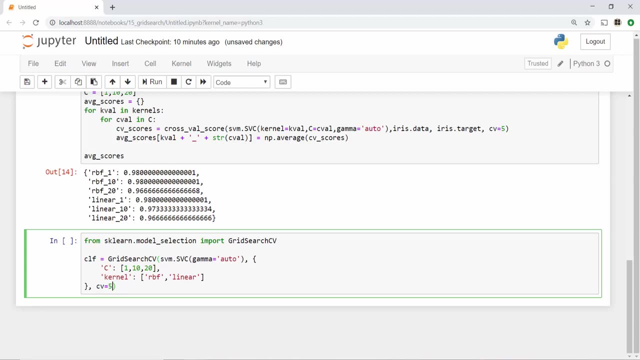 code blog convenient and we are writing the same thing in one line of code. okay, so cv is still using cross validation. okay, it's just that we are making this particular code blog. so cv is this: there is another value called return train score. if you, this is some parameter that. 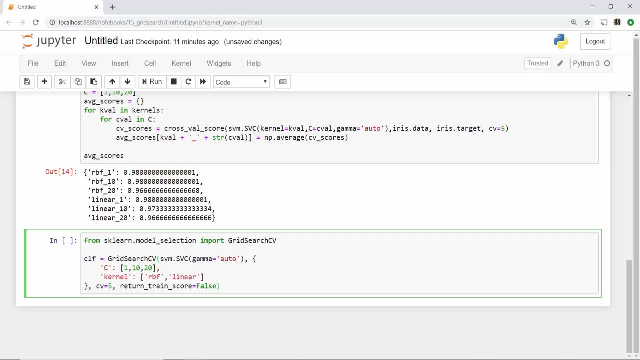 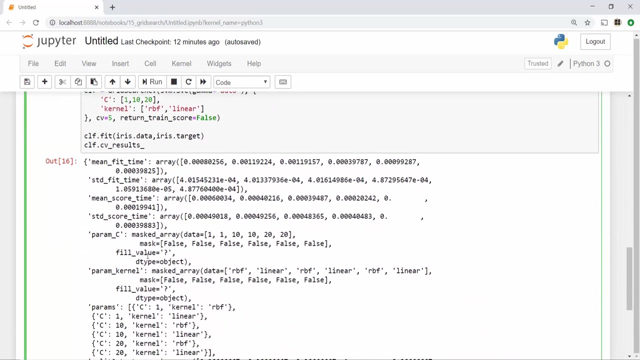 this method returns which we don't need. that's why we are saying: okay, it is false. once this is done, you will do model training by saying iris dot data and iris dot target. okay, and once that is done, we will print the cross validation results. when you execute this, you get these results now. if you look at these results, 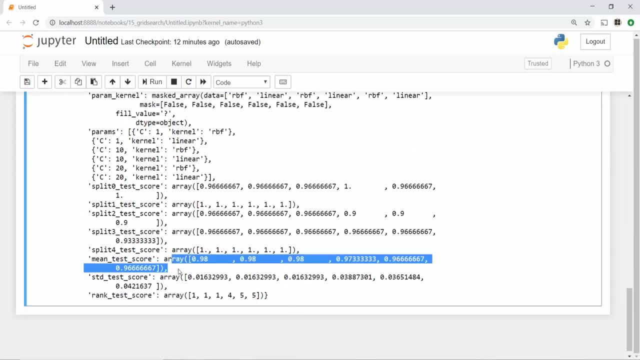 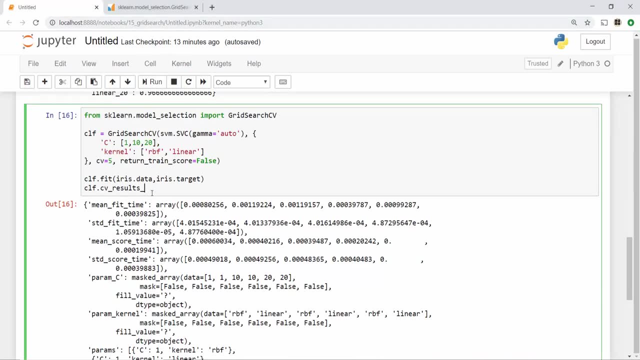 you will notice that you got this mean test score. cv results are not easy to view, but luckily sklearn provides a way to download these results into a data frame. here i have a skill and documentation and it says that this can be imported into panda's data frame. so that's the 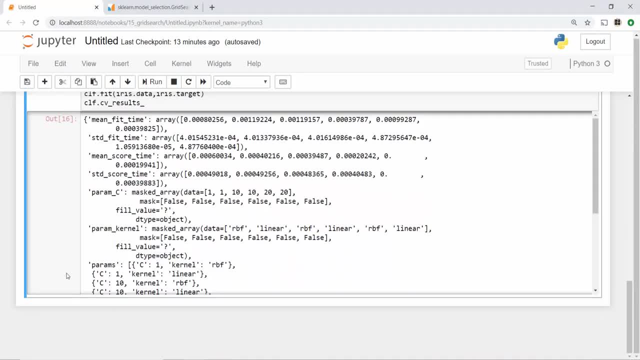 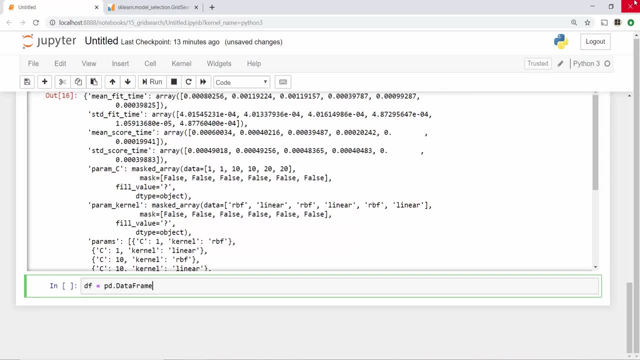 next thing i'm going to do, and all you guys are going to do, is i'm going to import this data frame here, just import the data there and copy this data in your đas electronically, and then i'm going to print it and i'm going to Divi and i'll just import it in fandasglich. so this: 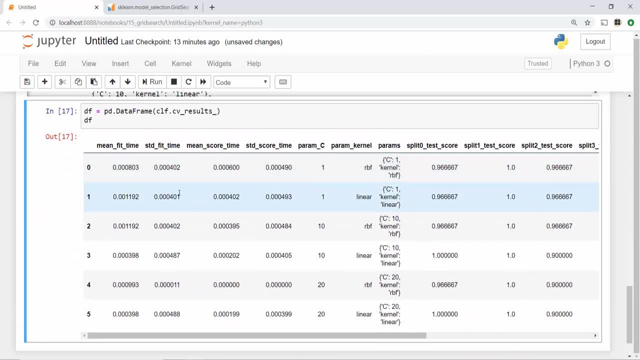 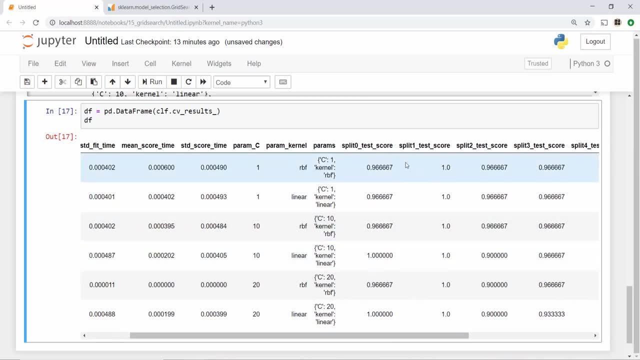 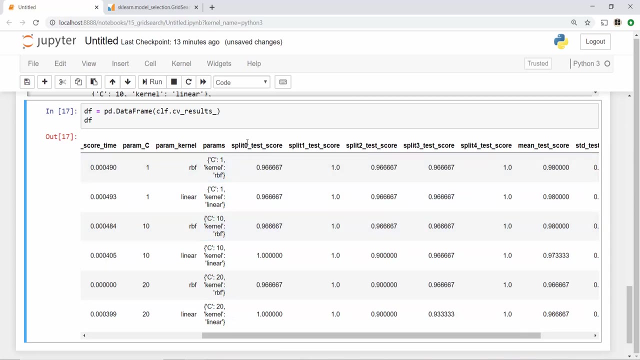 is going to Kate multi and it will divide by two. okay, next one, which is the mig field, and we'll put this link in the description over here and i'll just type it in the description: split. okay. we then five fold cross validation. that's why you get split zero to split four. 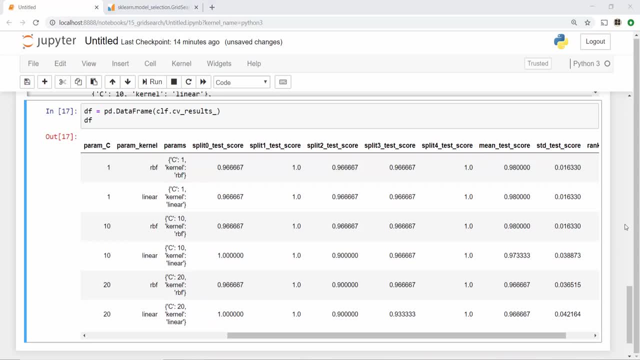 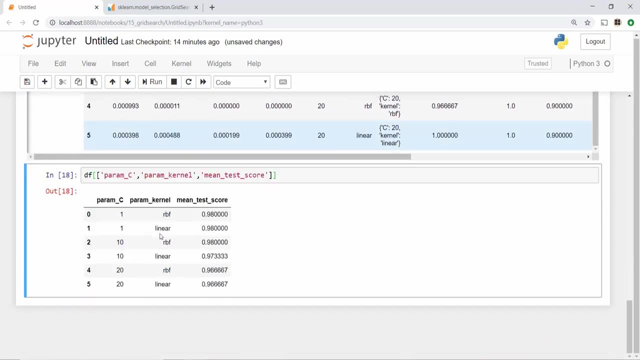 and then you have mean test score as well. some of these columns in this grid might not be useful, so i'm going to trim it down and just look at parameter values and mean score so you can see that these are the possible values of parameter c and then kernel, and these are the scores i got. 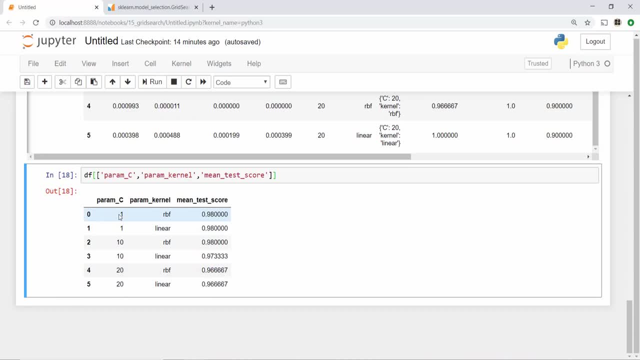 based on this, i can say that i can supply our first three values into my parameters to get the best performance. so we already did hyper tuning of these parameters. you see that this how this works right, and now you can have many, many parameters. all you have to do is supply them. 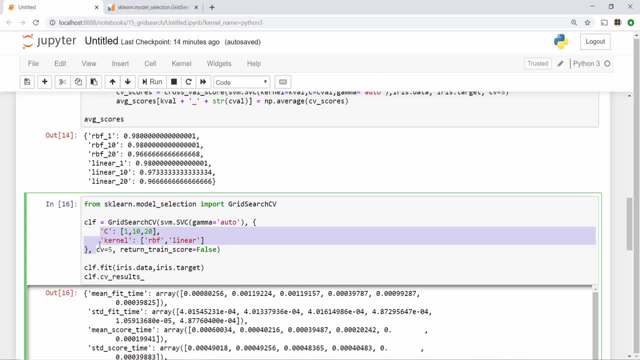 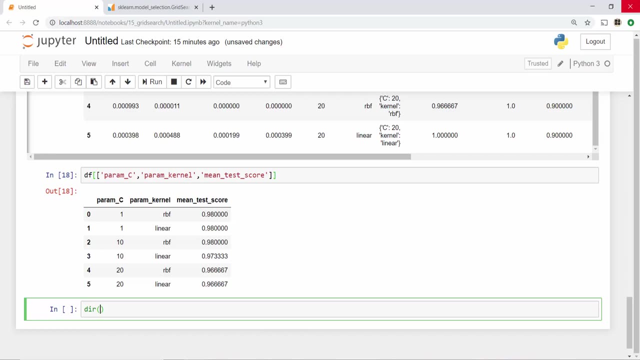 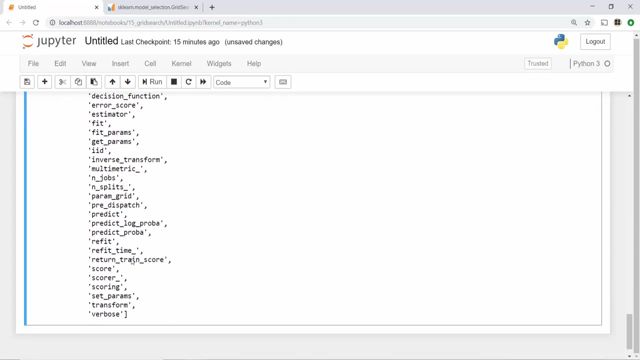 in parameter grid and this grid search cv will do permutation and combination of each of these parameters using k fold cross validation, and it will show you all the results in this nice pandas data frame. i can do dir on my classifier and see what other properties this object has, and i see some of the properties, such as based estimator. 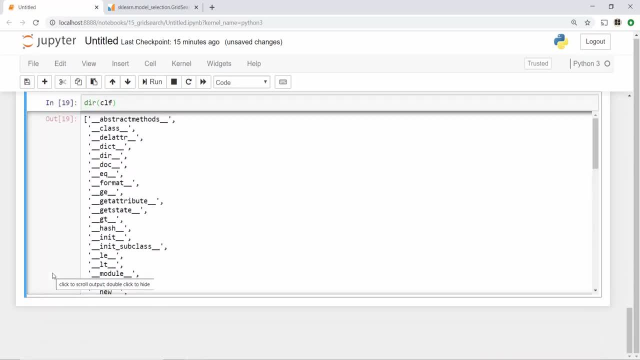 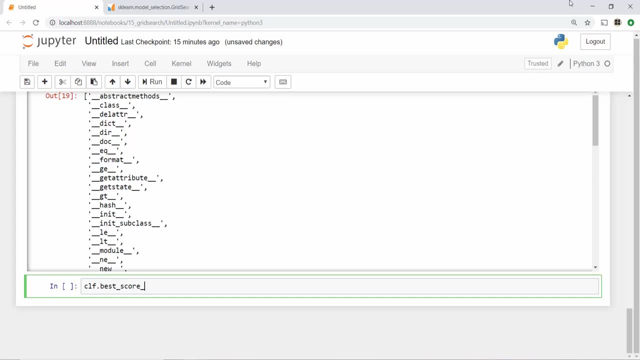 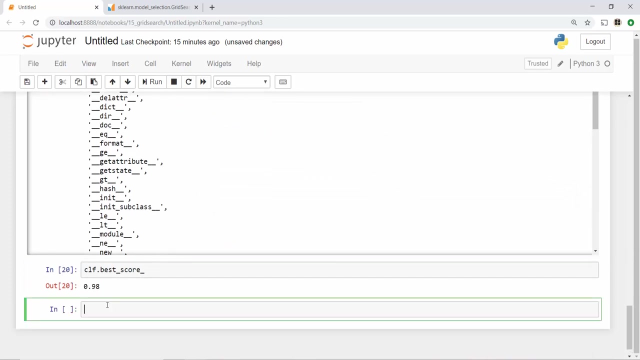 best params and based score. so let me try uh best score for. so, clf, the dot based score and the base score. it is saying 0.98, which is valid. see 0.98 is the base score. i can also do clf, dot, best params and it will tell me the best parameters in our case. 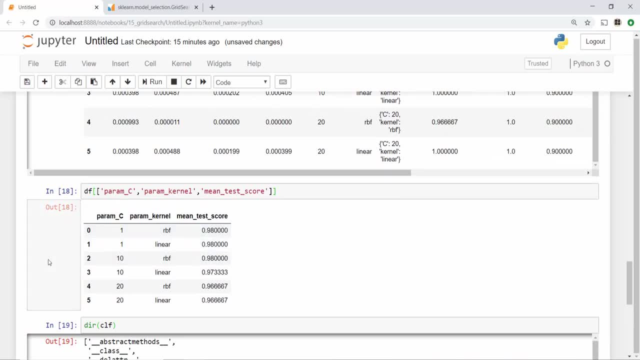 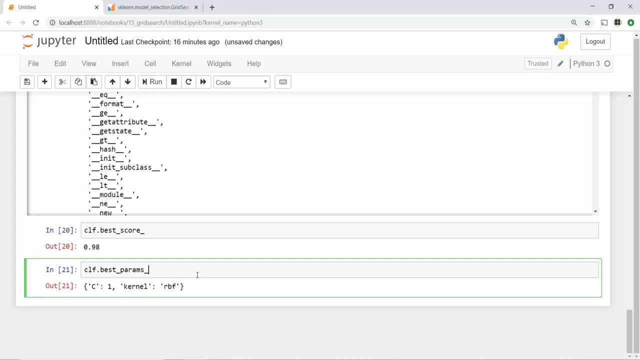 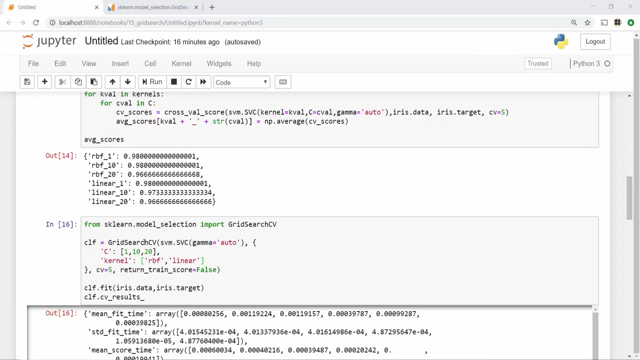 there are multiple parameters, which gives you optimal performance. but you can see the point. you just run grid search cv and then call based params to find out the base parameters, and these are the parameters you are going to use for your model. one issue that can happen with grid search cv is the computation cost. our data set right now is very limited, but just 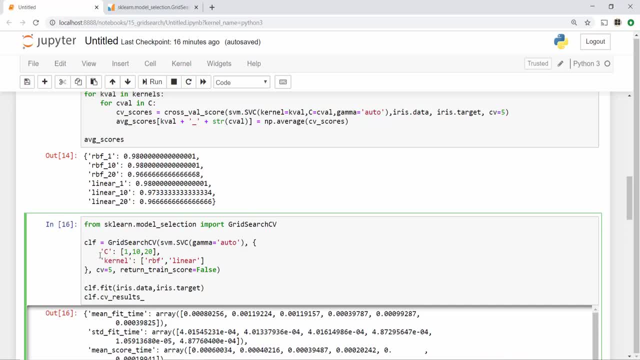 imagine you have millions of data points into your data set and then for parameters you have so many values, right now c values. i randomly took them to be 1 to 10. but what if i just want to try range, let's say number 1 to 50? okay, then my computation cost will go very high because this: 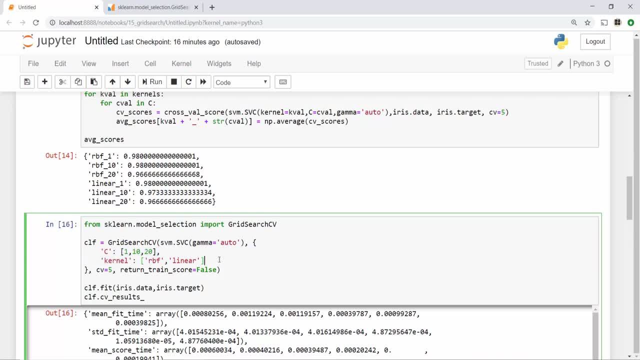 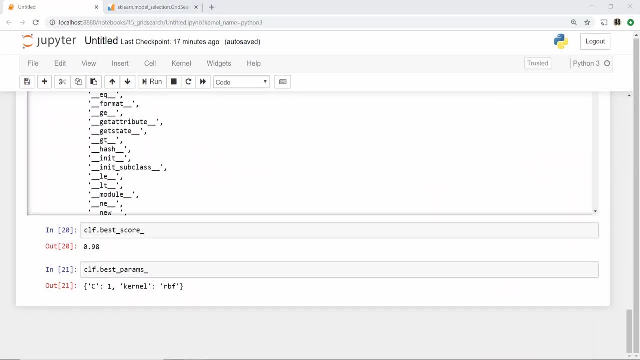 is a very high value, so i can easily try permutation and combination for every value in each of these parameters. to tackle this computation problem, sklearn library comes up with another class called randomized search cv. randomized search cv will not try every single permutation and combination of parameters, but it will try random combination of these parameter values and you can. 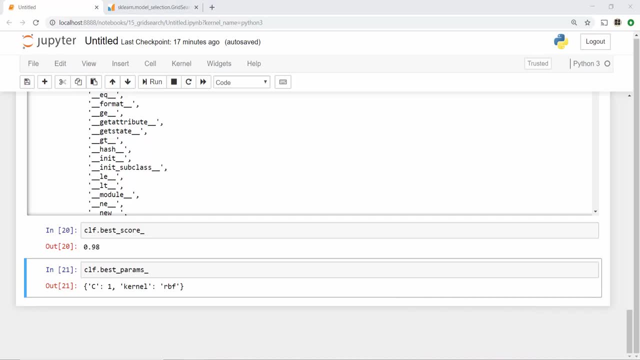 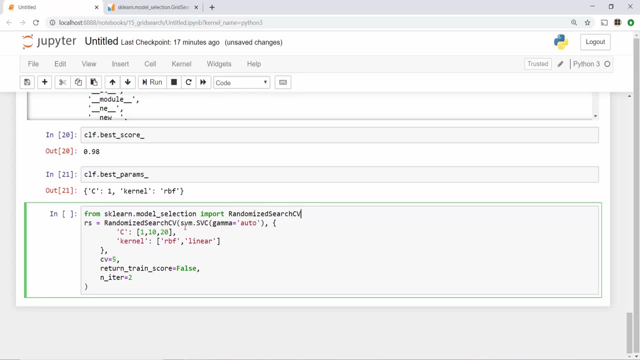 enjoy it with this 저에 mallürgen here. it allows you to try random mango combination. it works on all the parameters and this model is based on that- some of the parameters. this model is based on a multipleially choice simulation and that's exactly what dsk learned. 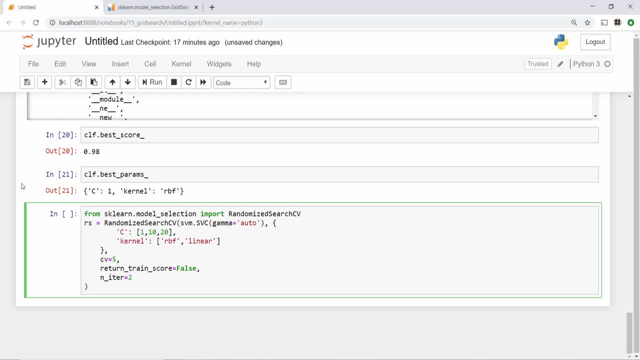 model, whereas this model is based on single method. so let's take a look. so dsk knows how it Works in this model. dsk is going to go through a process here and check it'll. Ochie For this model. you can see that we have three parameters: apiAndKnows, including dsk, value, aduy and dsk parameters at the screen. so you can see this can count for four supporting parameters and caused by a primary parameter than each parameter help. 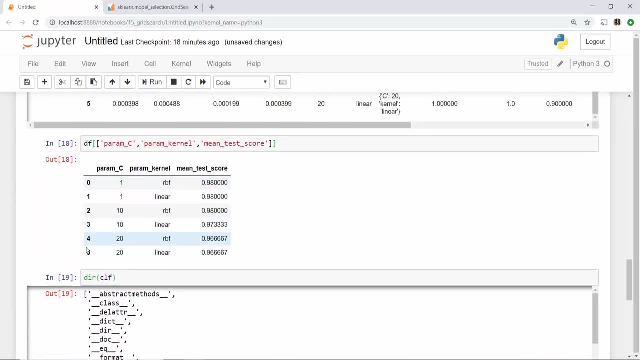 what Windows sql cod and the Mexican version TnS cv it. since you have that with Google all you can enable a Facebook application here at the local joshSheet. here we try total six. you see zero to five, so here it will try only two. 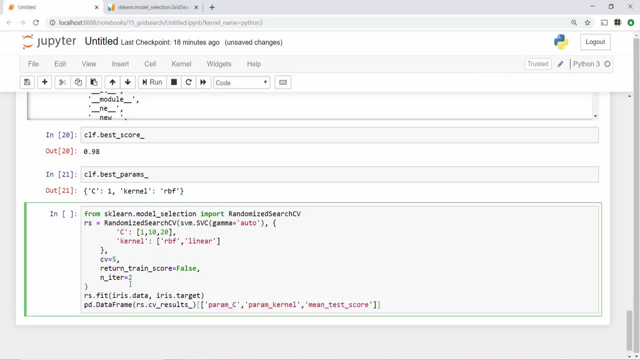 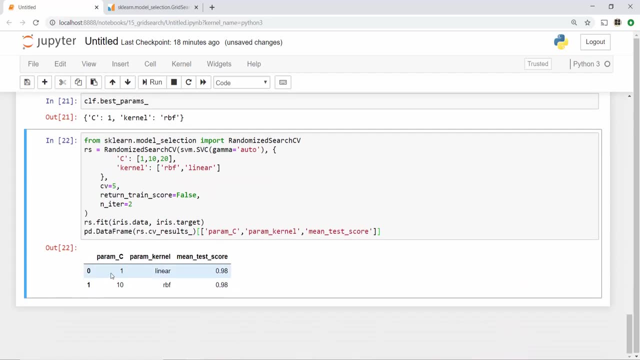 combinations and then we'll call fit method and then we will download the results into data frame. when I run this, you can see that it randomly tried C value to be 1 and 10 and then kernel value to be linear and RBF. when I run, 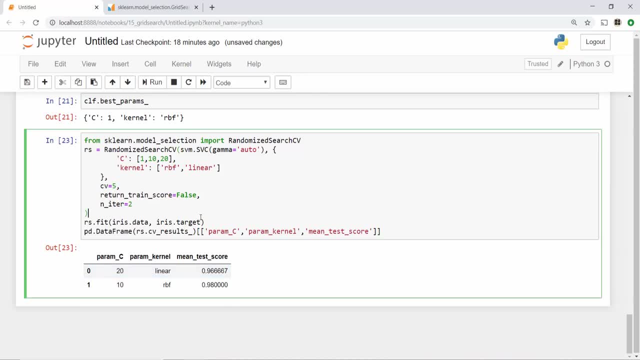 this again. it changed the value of C to be 20 and 10. this way it just randomly tries the values of C and kernel and it gives you the base score. this works well in practical life, because if you don't have too much computation power, then you. 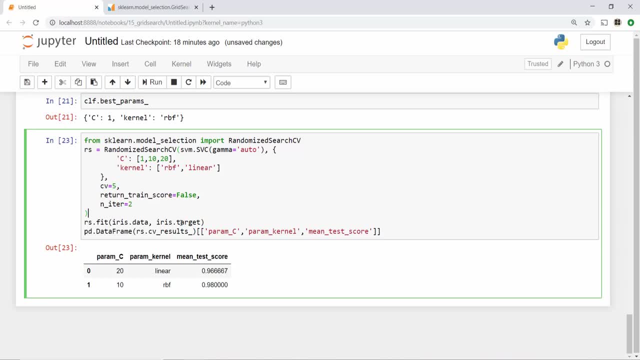 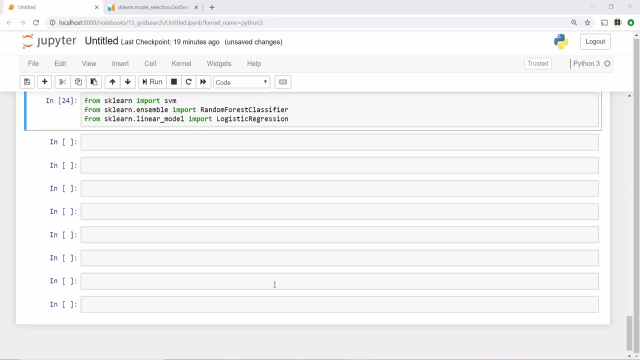 just want to try random values of parameters and just go with whatever comes out to be the best. all right, we looked into hyper parameter tuning. now I want to show you how do you choose a based model and how do you choose a base model. and how do you choose a base model. 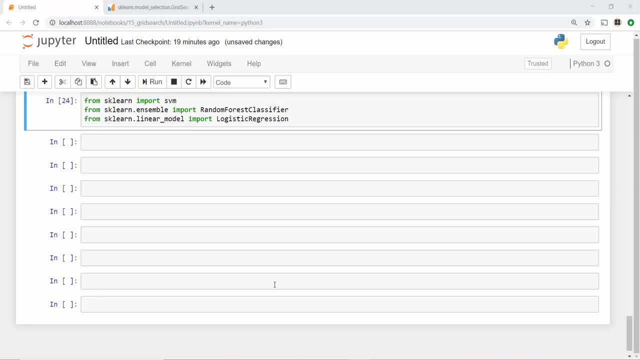 for your given problem for our iris data set. I'm going to try these two classifiers, okay, SVM, random forest and the logistic regression, and I want to figure out which one gives me the best performance. you have to define your parameter grid and I'm just defining them as a simple JSON object or simple. 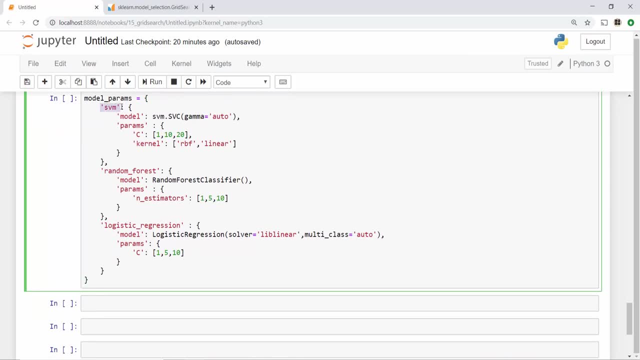 Python dictionary where I'm saying I want to try SVM model with these parameters, random forest with these other parameters. I want the tree value of random forest to be 1, 5 and 10 and this n estimator is an argument in random forest classifier. okay. similarly, the value C is an 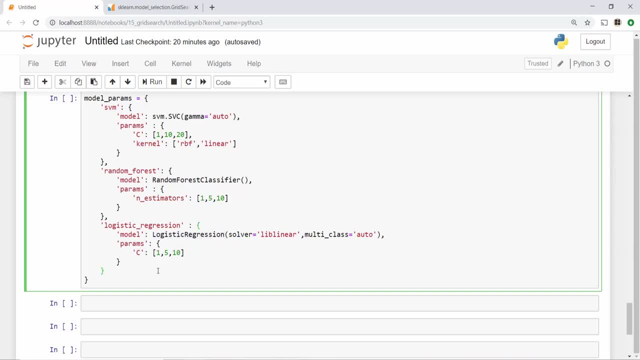 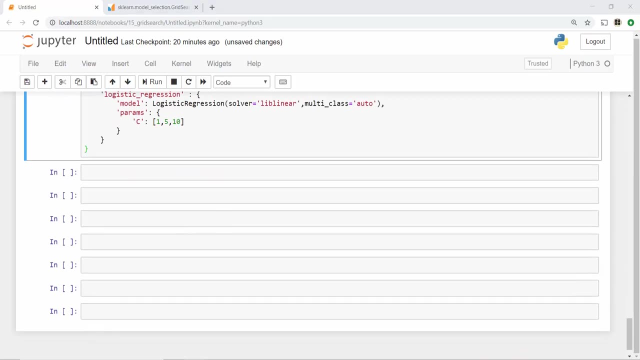 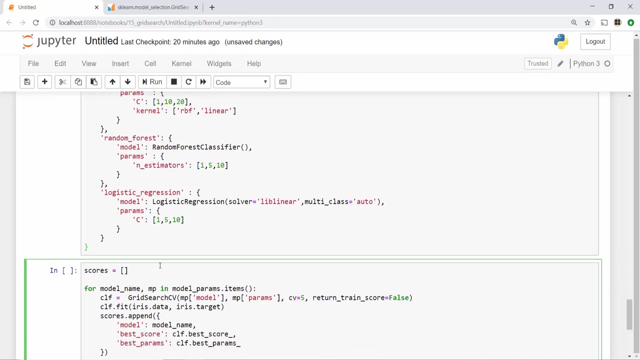 argument or a parameter in logistic regression classifier. once I have initialized this dictionary, I can write a simple for loop, so I'm just going to show you that for loop here. and this for loop is doing nothing, but it's just going through this dictionary values and for each of the values it will use grid. 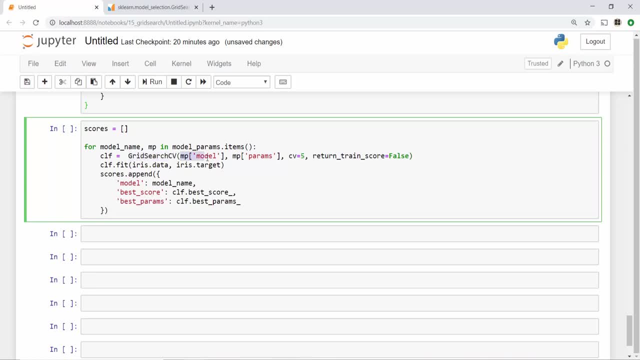 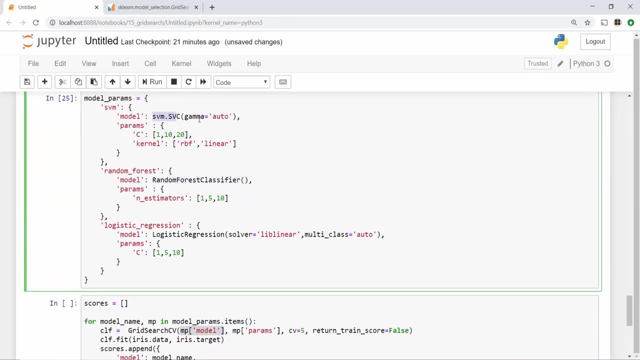 search CV. so you can see that. the grid search CV. the first argument is the classifier, which is your model. so here you can see the model is classifier. so it is trying each of these classifiers one by one with the corresponding parameter grid that I have specified in this dictionary. you can see that. 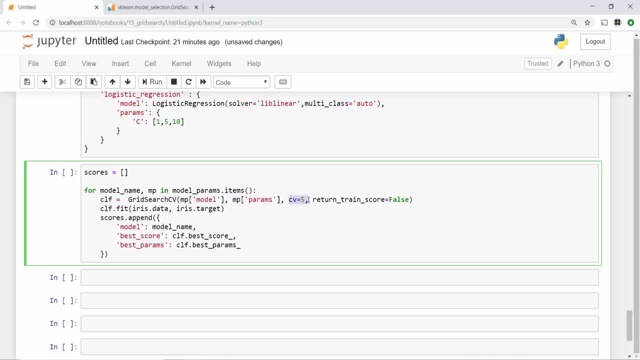 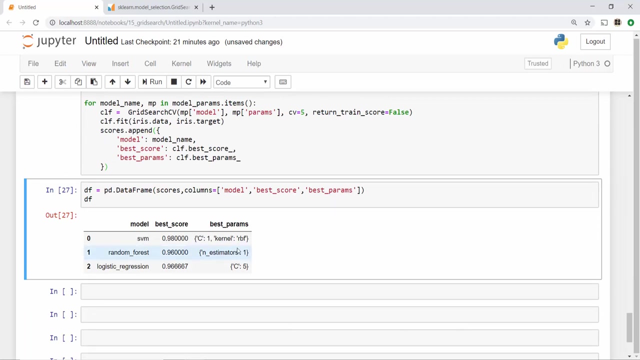 parameter is the second object, second argument, and then classifier: addition is 5i. then run my training and then append the scores into this course list. when I run this, my scores list has all those values and all I'm going to do now is convert those results into pandas data frame. when I do,